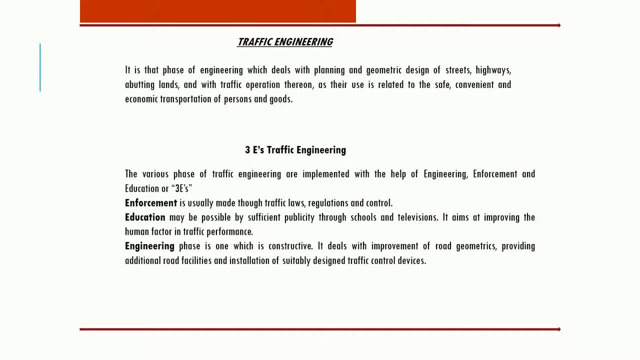 it is that phase of the engineering which deals with the planning and geometric design of street, highway and about the lands and with traffic operation theorem. normally in case of traffic engineering we are using irc rules and regulations, that is, indian road congress, which has been introduced in 1934. so as per the recommendations, we have some rules which come under this traffic. 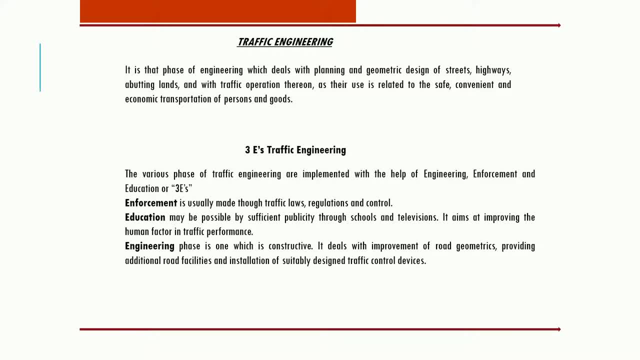 engineering in. one of the important point, that is, three, is of traffic engineering, which is normally related with our psychology, the student. what do you mean by three is of traffic engineering and how these are important. basically, these three is include in for enforcement, education and engineering. so let's discuss about the enforcement. 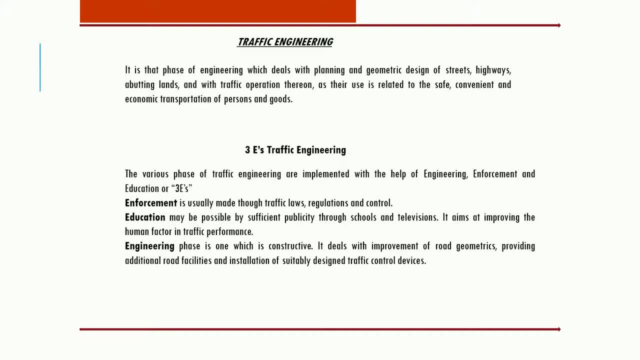 basically, enforcement is usually made through the traffic laws, regulations and control where, being a road user, we should follow all the traffic rules and regulations. so following these rules and regulation is the part of enforcement. education may be possible by sufficient publicity through school and television and its aim at improving the human factor in traffic. 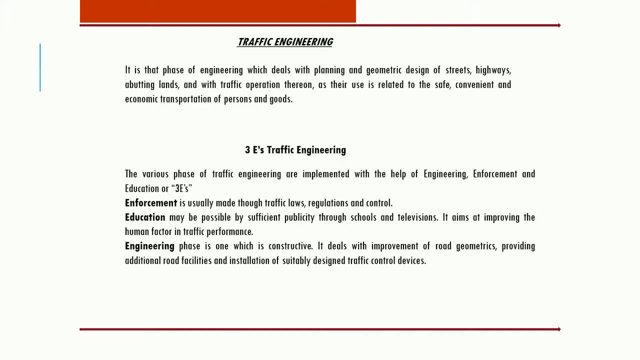 performance. we know that, or when i was in school, there are many programs was conducted which are related with the awareness regarding the road users, regarding to the road usings, awareness about the traffic engineering. so this education is very important. first, we should educate about the tra, various traffic rules and regulation, and we should forward all this information to other. 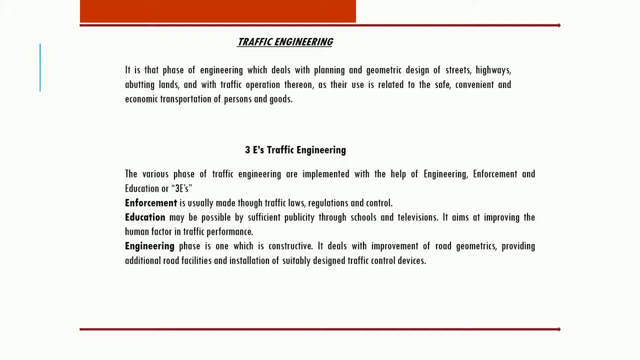 people so that every can follow this traffic rules and this way we can avoid the accidents and there will be the proper awareness regarding this traffic engineering. the third point is engineering. we know that engineering is play very important role for the design, construction and maintenance of the highways and others- roadways, basically. 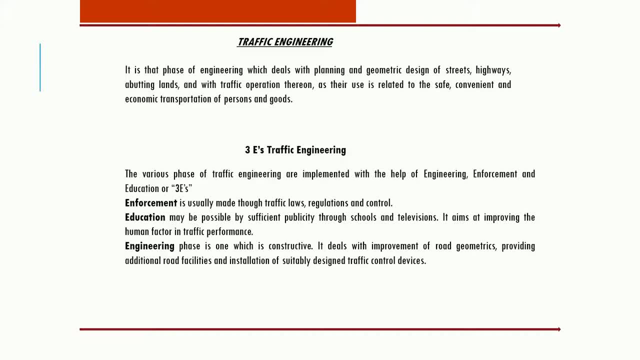 it is also deal with the improvement of road geometry. we can providing additional road facility and installation of suitability design, traffic control devices. so one person should have the engineering knowledge. he can use that engineering knowledge for the construction of the road. so this way, this three is are very important, which include enforcement, education and engineering. 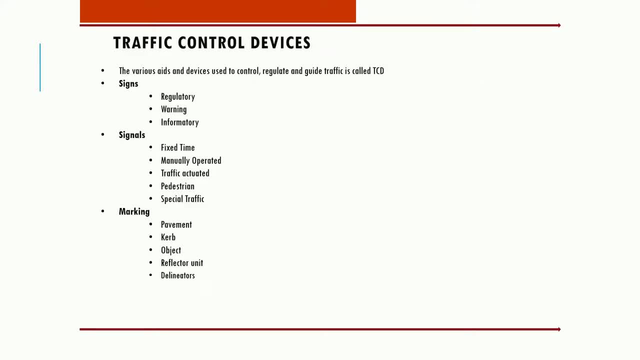 now, students, we are going to discuss about the traffic control devices. basically, if we have to follow some rules and regulations, so in that case there are some devices that should be used and we all are know that we are familiar with these devices. so this device includes first signs when you are moving on the roads we can find. 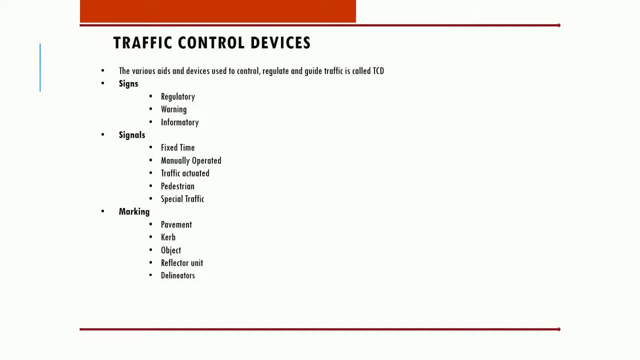 the various types of signs are there which are useful and which give the information to the road user. so this sign include the a regular type of sign. for example, turn right, turn left, go straight. these are the regular type of sign. some warning signs will be there. the railway tracks is in forward. 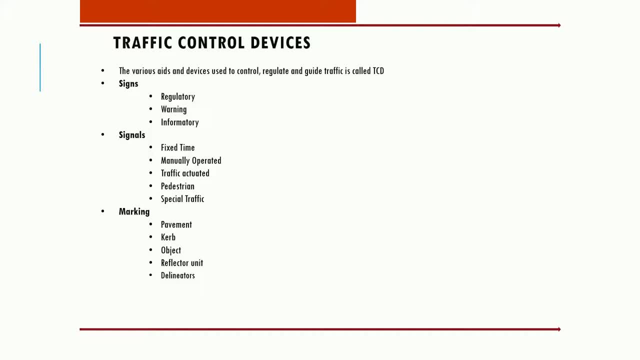 direction: school is ahead. reduce the speed of your vehicles, go slow. children's are there. so when we are finding this type of signs on the road, then it is called as the warning type of sign and some are the information type, like medical or hospital is ahead, petrol pump is ahead, school is ahead. 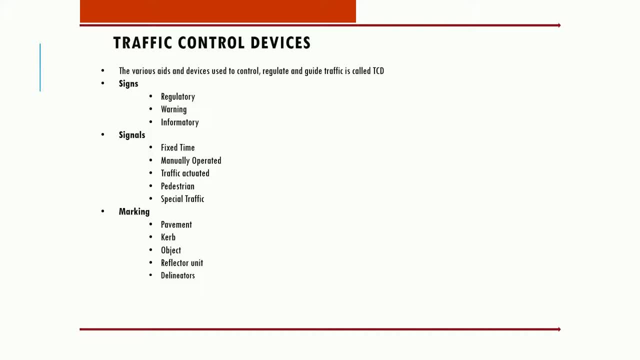 hotel is ahead. many time we are finding this type of signs are on the road. so all these signs are come under the informative type. so basically there are three type of sign. one is regulatory, warning and informative, and then we also know about the signals. basically we have seen three type of signals: road, 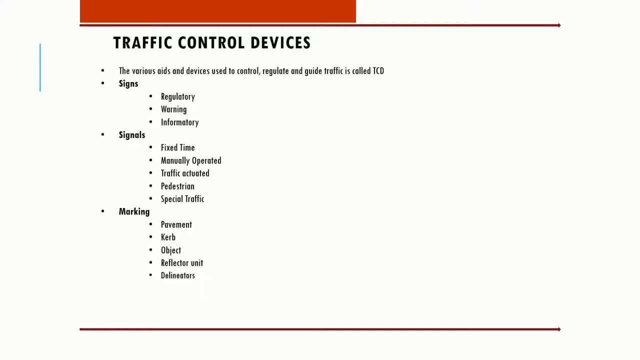 signal. one is red, second one is green and third one is yellow. so they all are called the fixed type of signals. there are some manually operated signal, traffic accurate signals, penetration signals and special traffic signals. when we are moving on the road, we have find various types of marking on the road. 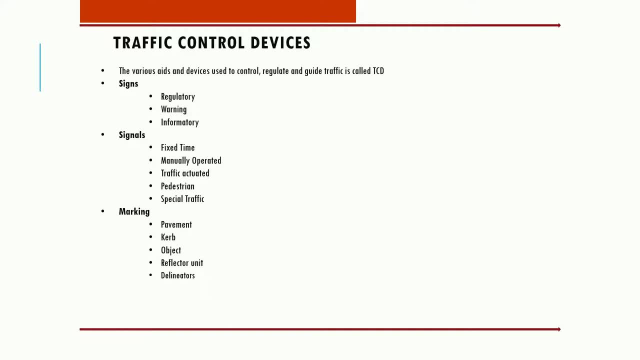 this marking or the pavement marking, top marking, object marking, reflector units and delineators. basically we are using all this type of marking for the informative, the person those are using this road, the driver should get some indication, he should get some information so that there will not be any type of accident. so in that case we are using 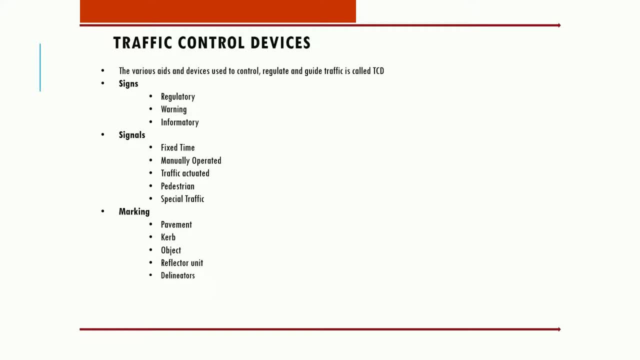 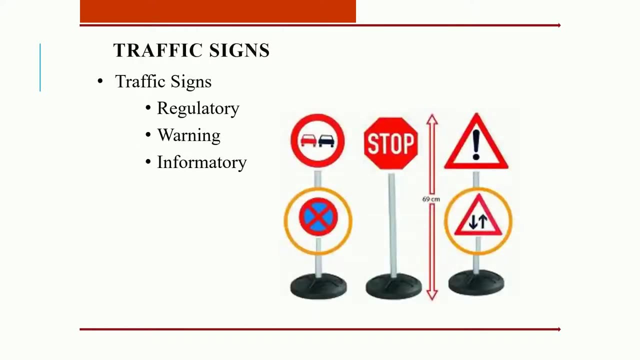 this type of marking. we always see some white colors and yellow color strips on the roads. so all the steps were using for the as a informative marking which give the information to the road user. so you can see already I discussed that these are the three traffic signs where you can see how 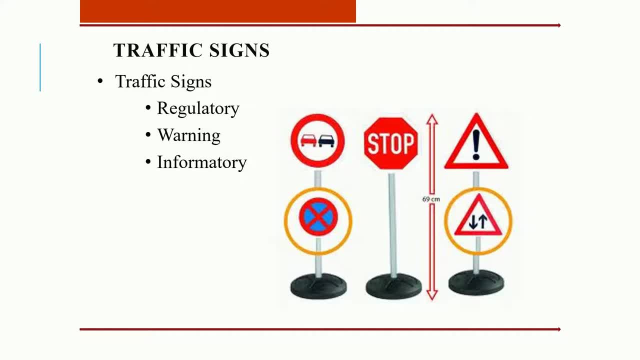 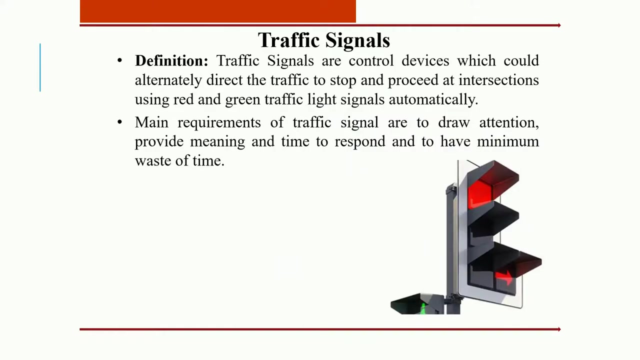 they are indicated, various regulations, warning and informations, and all these are important that drivers or road users can get the information and all this type of information is comfortable and one can drive safely on the road. and this is familiar, or all you are familiar with the various type of traffic signals, the 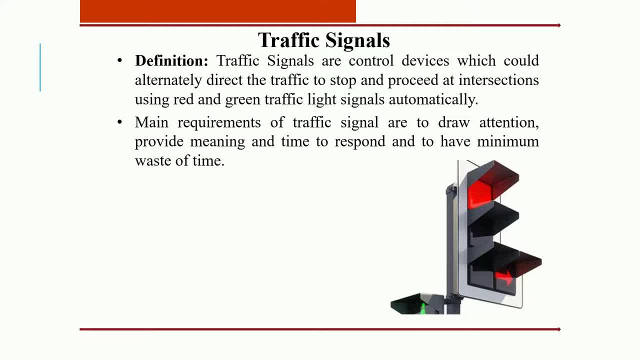 traffic signal of control devices which could be, alternatively, direct the traffic to stop and proceed at intersection using the red, green traffic light signals automatically. the main requirement of traffic signals are to draw attention, provide meaning and time to respond and to have a minimumungen restop time. so, in regards to our safety, this traffic signals is 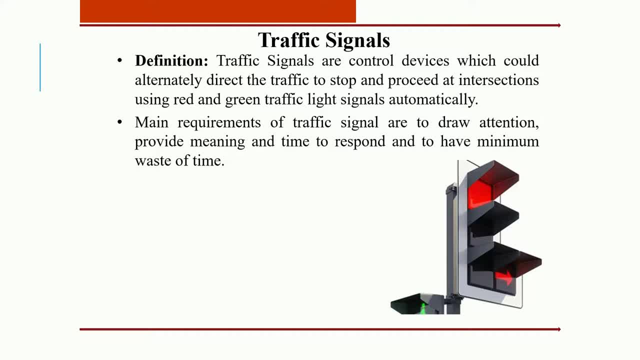 lated to зависYeah, so all you need to do is plays an important role. basically, there are three type of signal. one is red, second one is green and third one is blue. we know that red indicate that one should take the responsibility of stop the grid, indicate you can move and 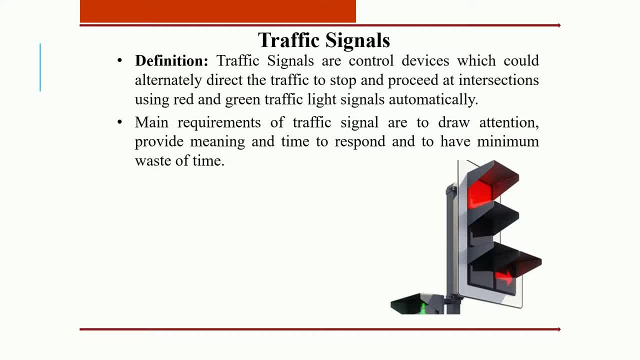 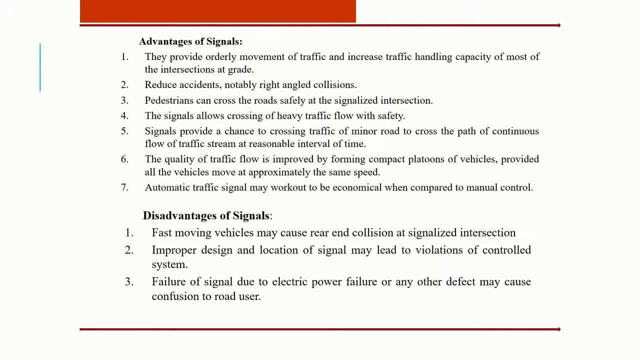 yellow indicate that you should be ready for moving. so everyone should follow this traffic signals so that we can, overall, avoid the various types of accident on the road. there are some advantages of signal as well as some disadvantage. what are the advantages of the signals? they provide early movement. 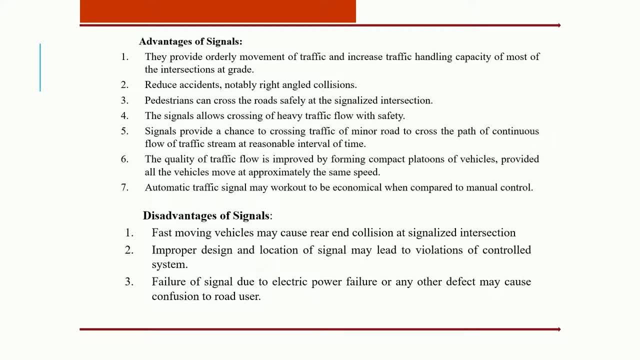 of traffic and increase the traffic handling capacity of most of the accidents at the grid. it reduce the accident, notably right angle collisions. pedestrians can across the road safety at the horizontal intersection. the signal allows crossing of heavy traffic flow with safety signal provide a chance to crossing traffic of minor road to cross the path. 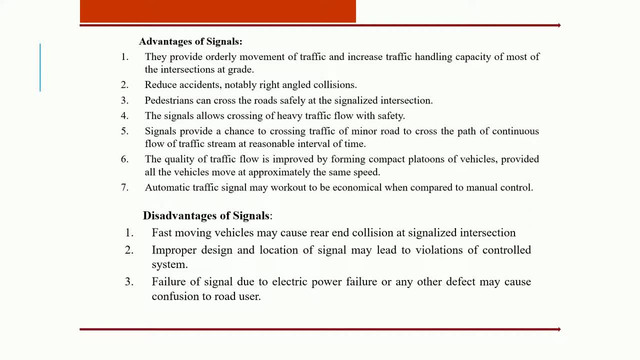 of continuous flow of traffic stream at a reasonable interval of traffic time time. The quality of traffic flow is improved by forming compact platoons of vehicles, providing all the vehicles move at approximately the same speed. Automatic traffic signals may work out to be economical when compared to manual control. 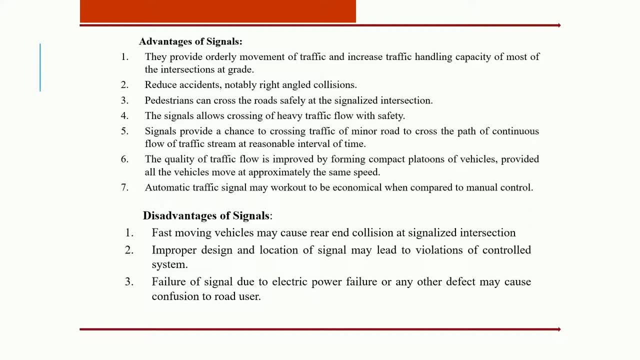 Then what are the various disadvantages of signals? Fast moving vehicles may cause rear and collision at signalized intersection. Improper design and location of signal may lead to violation of control system. Failure of signal due to electric power failure or any other defect may cause confusion to the 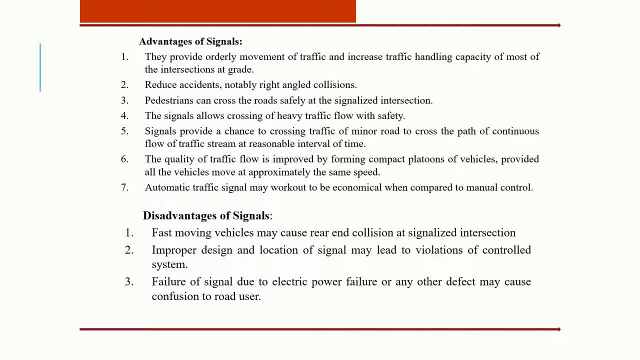 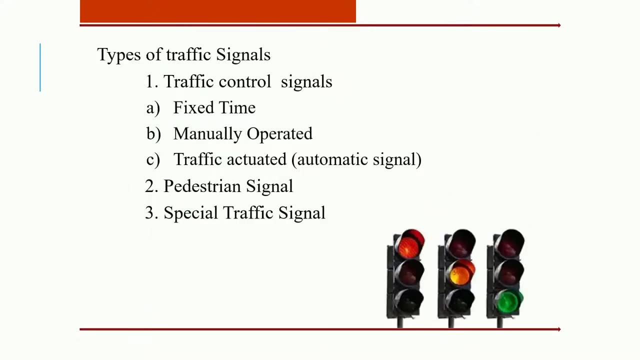 road users. So these are the some disadvantages of signal and while following this various road signal, we should consider all these advantages and disadvantages. What are the various types of the traffic signal? So first is traffic control signal, which include the fixed time signals, manual operated signals, automatic type of signals. 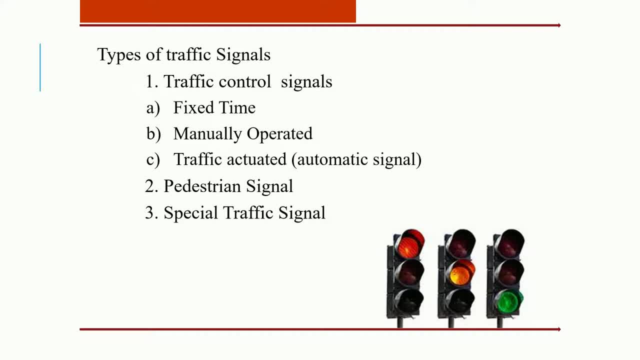 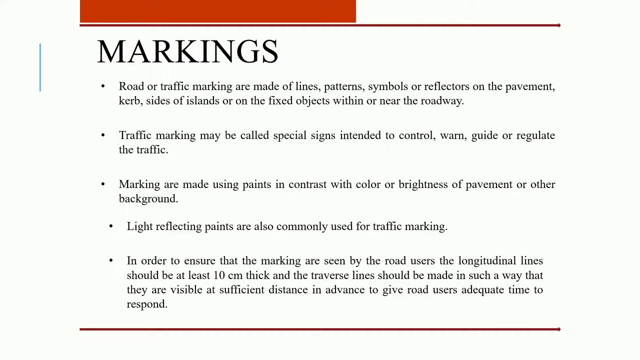 penetration signals. penetration means those people, those are using the road, that type of people and special traffic signal. These are the various types of the signal and, as per the requirement of the location, we are using these signals. We also discussed about the marking and for giving the various information and to 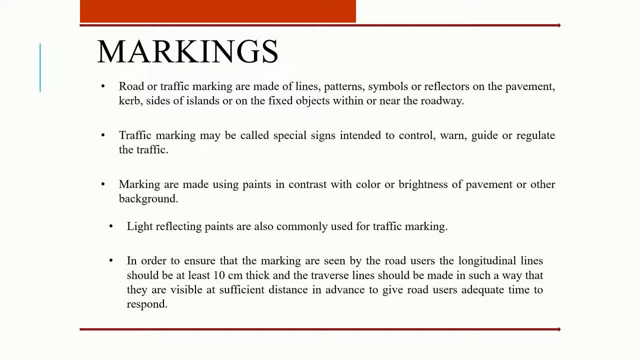 avoid the any type of collisions on the road marking plays a very important role. The road or traffic marking are made up of line, pattern, symbol or reflector on the pavement curbs side of the island or on the fixed object within or near the roadways. 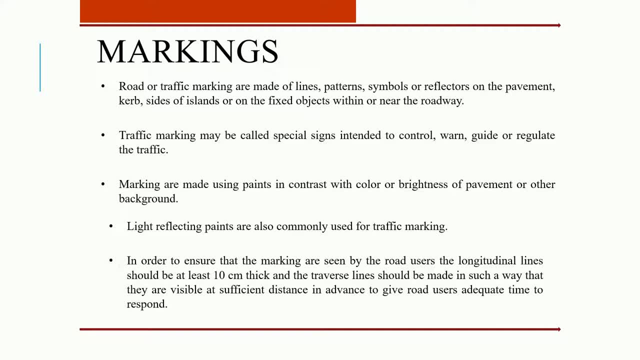 and I hope you all are seeing various types of yellow and white type of marking on the road. The traffic marking may be called special sign. The traffic marking is a kind of marking that is used to guide or control the traffic. Basically, this marking is useful to guide and regulate the traffic. 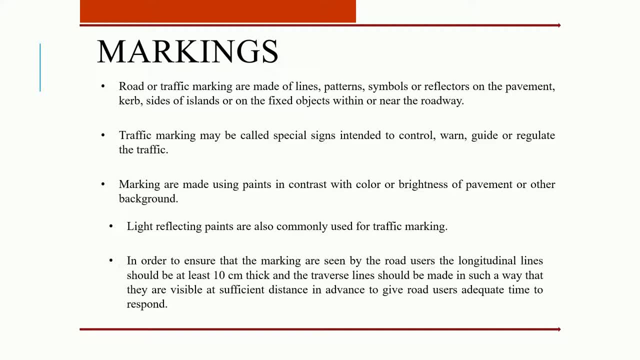 Marking are made using the paint in contrast with the color or brightness of the pavement or other background. Contrast with the color is very important with the background, otherwise it will not be clearly visible to the road user. Light reflecting panes are also commonly used for the traffic marking. 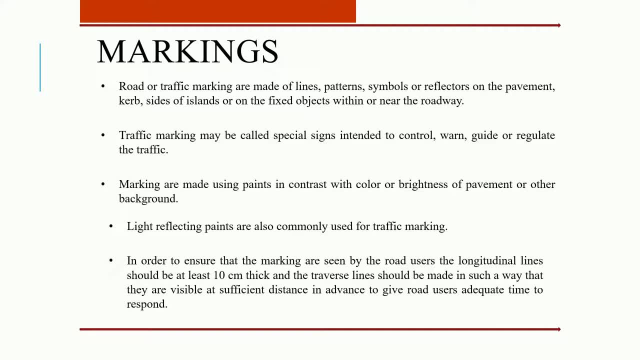 In order to ensure the markings are seen by the road user, the longitudinal line should at least 10 cm thick, and traverse lines should be made in such a way that they are visible at sufficient distance in advance to give road user adequate time to respond. 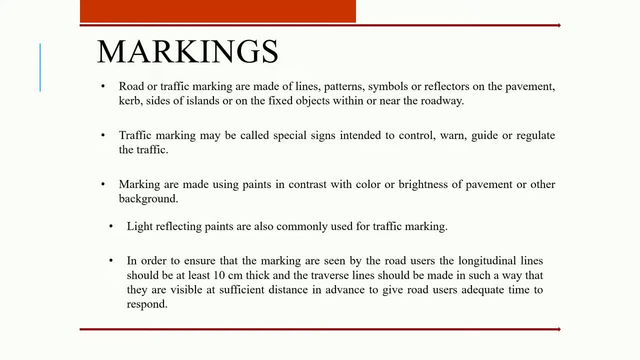 So when you are using this marking, it should have a particular type of thickness, otherwise there will be the less visibility of this type of patterns on the road and it will be harmful for the road users. So if someone wants a safe and comfort ride on the road, so everyone should follow this. 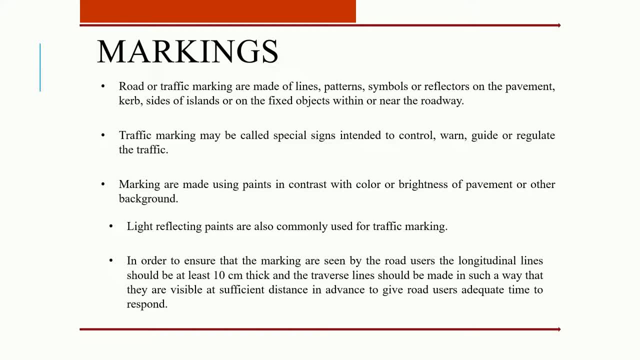 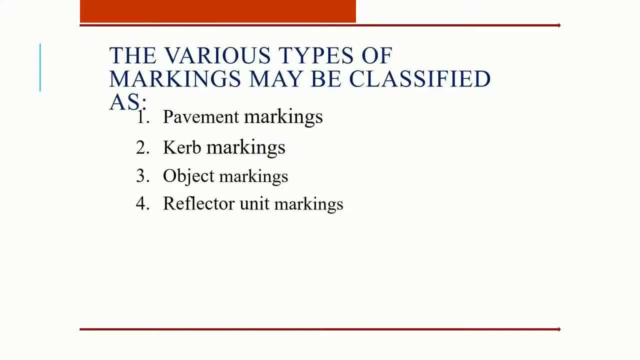 type of marking and follow all the rules and regulations of traffic, that we can reduce the various types of accident. Now there is a classification of various types of marking and they can be classified as a pavement type of marking. We know that there are two type. 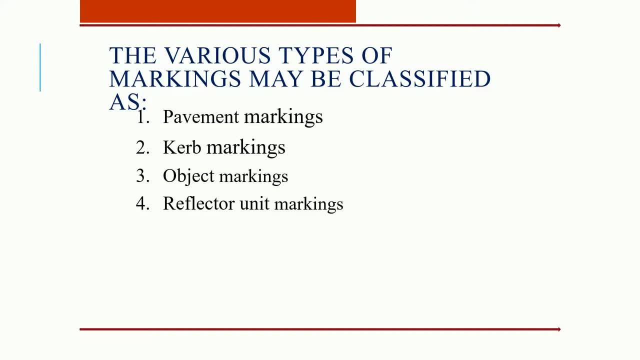 of pavement. one is the rigid pavement and second one is the flexible pavements. So the marking, those we are using on the pavement, is called as the pavement type of marking: Curb marking, object marking, reflector, unit marking. these are the various types of marking, those we are using. 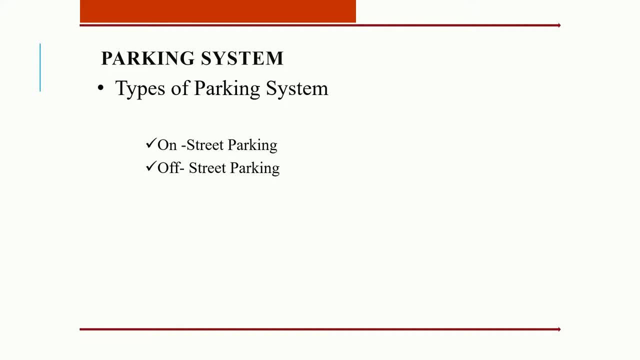 Now the next point, and already we have seen today in the videos regarding to the parking system. Basically, there are two important parking system. one is the on-street parking system and second one is the off-street parking. So basically in last class, I have shown you video regarding to this: on-street parking and off-street. 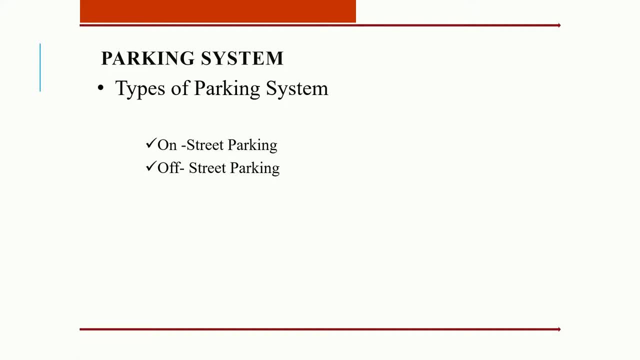 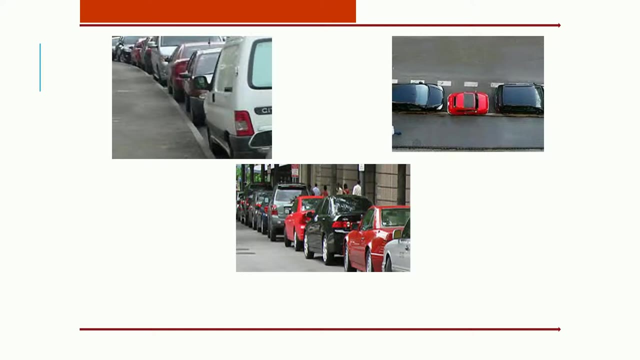 parking and I hope you have understand how this parking are important as per the locations and site. So, student, here you can see these are the various types of parking. the various types of cars are there on the road And at this side of cars you can see various types of marking with. 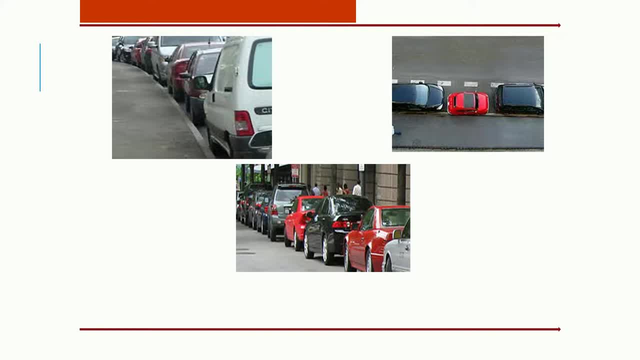 the white color. at some spot- these are the complete white line- is there, or at some part there is a dotted white line. So when you find this type of parking on the road, this type of parking is called as the on-street parking. Now, those days, people use roads Also as the non-terminal systems. 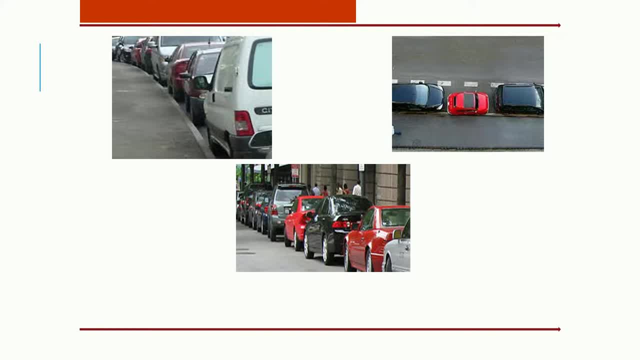 parking we are. we have some provision on the road and we are providing some space on the road which can be used for the parking. so that is called as the on street parking. and in on street parking all the vehicles are parked behind to each other. you can see in these pictures. this is called as 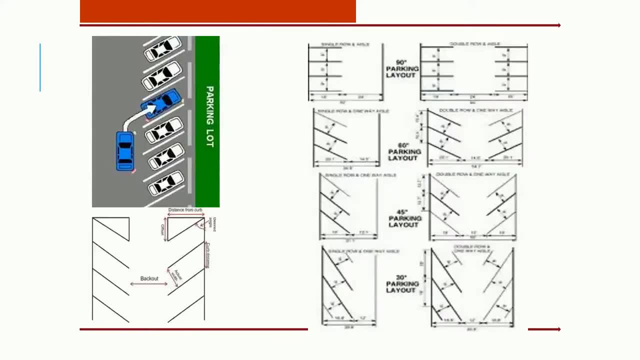 the on street parking. uh, this is another type of parking. so here you can see, i can see some car car park inclined to each other. so there are various types of parking layout. when we park the vehicles in 45 degree, 60 degree or 90 degree, then it is called as the various. 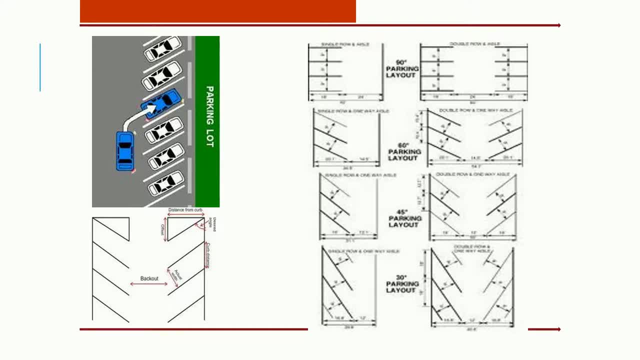 slot or pattern. so in first figure you can see all the vehicles are parked to each other in 90 degree. in second figure you can see these vehicles are parked at an angle of 60 degree. in third you can see the vehicles are parked at angle of 45 degree and in last figure you can see it is parked 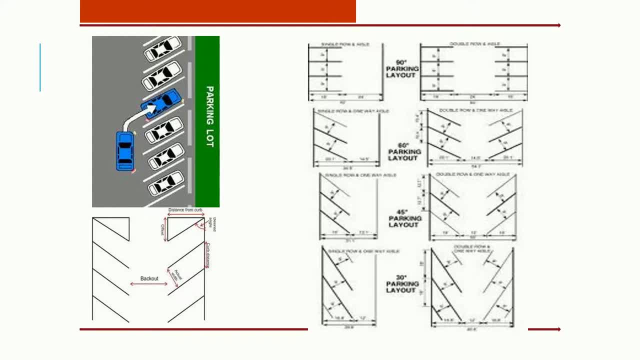 at an angle of 30 degree and left side one colored for photo is shown where you can see various uh parking slot which is normally used for the road parking, and these are very uh useful because in that case we can minimize the space and maximum car or vehicles can be parked on the road. 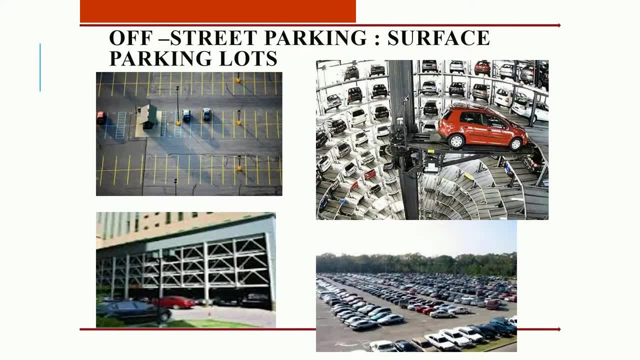 this is the another picture, uh, where you can see the various off-street parking. uh, it may call at the surface type of parking slot. so in first figure there are parking slots and by being you can park your vehicles here. in second figure you can see this is the modern type of parking. 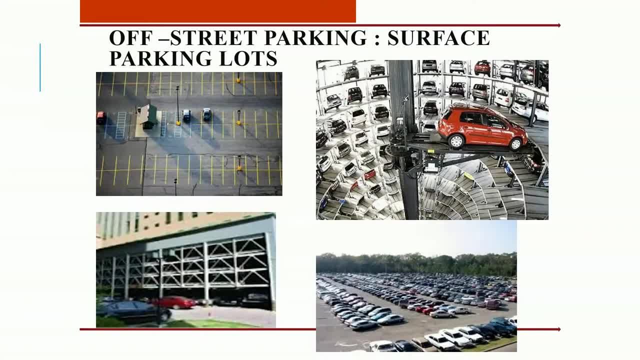 and, like it, flowers and sea show in the background. also, if you see, there will be a″″†″ reveal when you nearly zero in the″″‡‡‡‡‡‡‡‡‡‡‡‡‡‡‡‡‡‡‡‡‡‡‡‡‡‡‡‡‡‡‡‡‡‡‡‡‡‡‡‡‡‡‡‡‡‡‡‡‡‡‡‡‡‡ reflex. 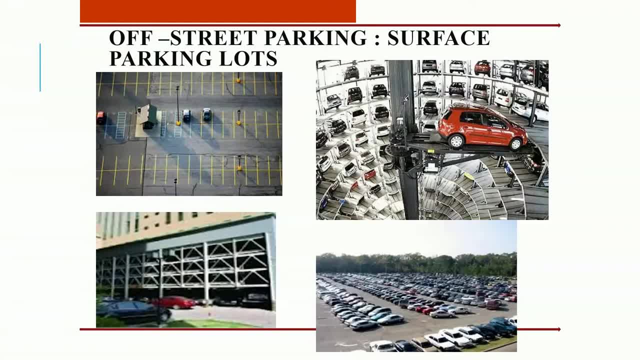 show like the have 23 fields shown um. here you can see one vehicle has parking space. so within that advantage three note: And when we are providing this type of parking. so in that case the person will get the comfort that he has parked his vehicle on the safe side. 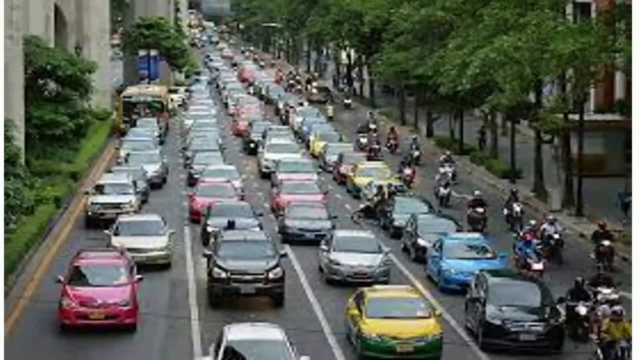 I have taken some pictures from other countries So you can see here. these are the various slots which are available on the road where there are many vehicles are parked in behind to each other. So this is one of the pattern. on this pattern you can park the vehicles on the road And in right side you can see the other vehicles can move. 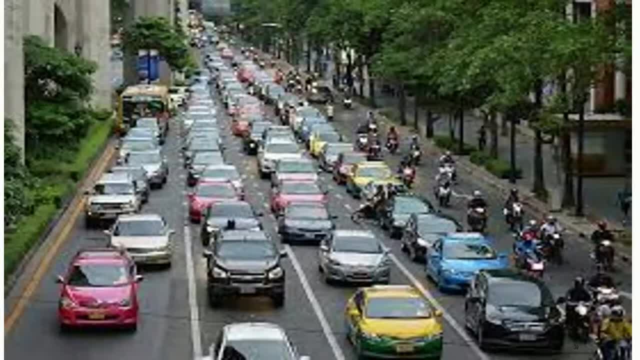 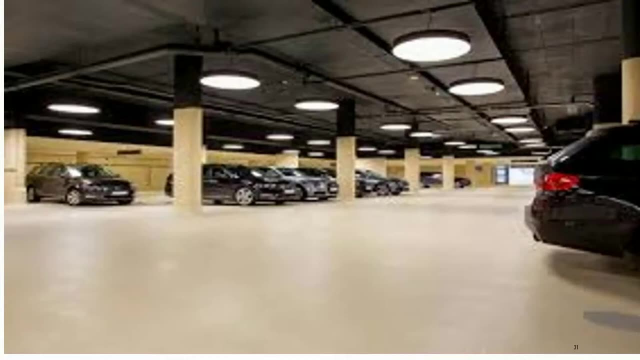 So it is a big lane. So here near about four lanes are provided for the parking And in last lane there is a movements of traffic. You can see in this picture. this is a underground type of parking. So here various slot has been provided as a parking area. 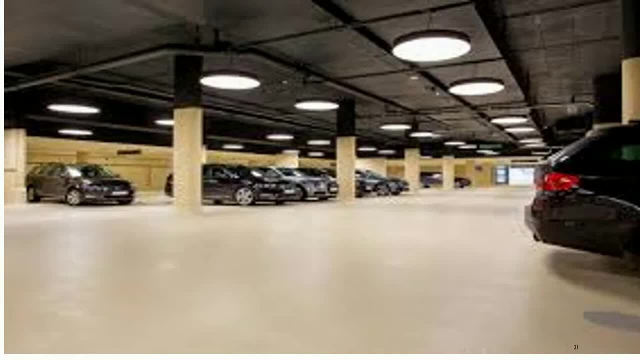 Here you can see all the cars. So the cars or vehicles are parked properly and various types of ventilations and lightings are provided on this point. So when there is a this type of parking, so one can say that this vehicle is safe. 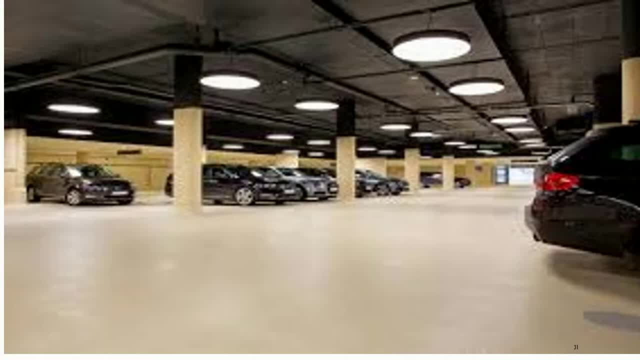 And this way or this type of parking is normally available in various big mall or big industries, And this way or this type of parking is normally available in various big mall or big industries and when we are doing this type of off-street parking so we can reduce the traffic volume. 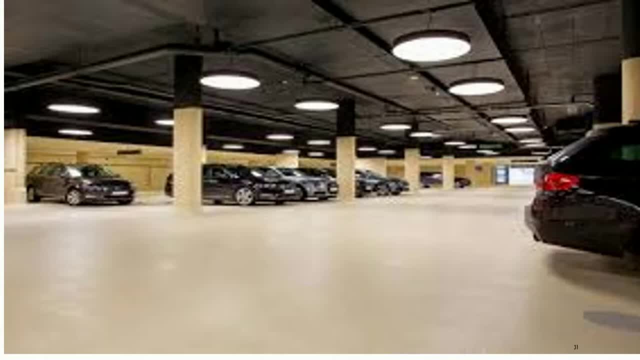 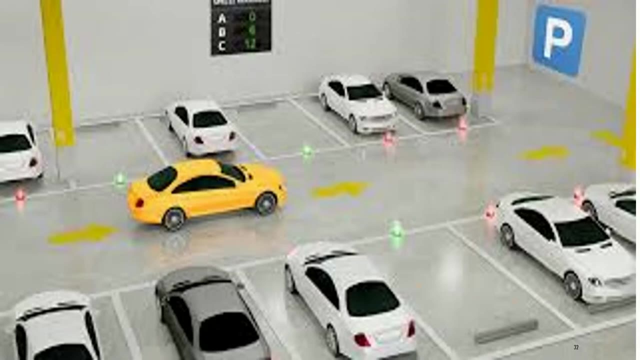 on the road and it is a safer type of parking. nowadays, in metro countries, in metro cities, we are providing this type of part parking. this may be surface parking or underground parking is also uh here you can see. uh, these are the various uh parking slots are provided. 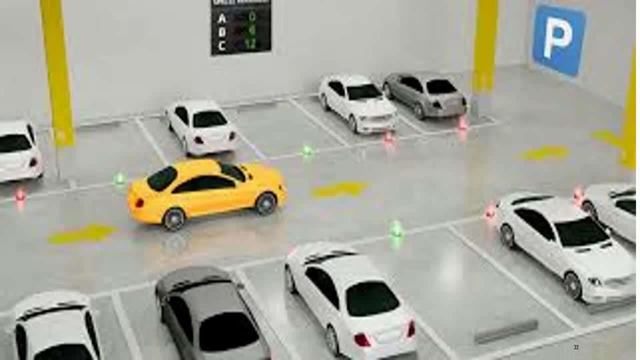 here, one portion has been allotted for the car parking and everyone can get a separate slot where he can park his vehicle and once parking our vehicles in the in that type of way. so in that case we can understand that this is to the safer side. nowadays in india we are using this various types of parking slot in. 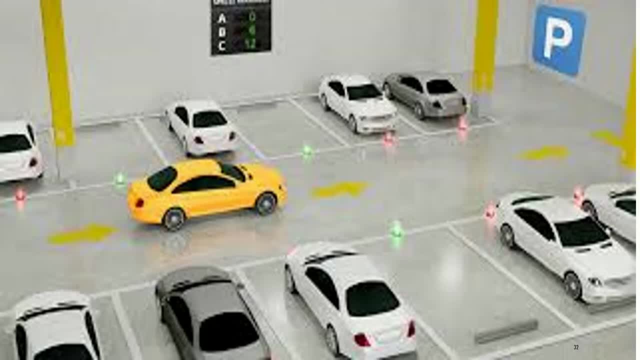 malls we are using this type of parking slot on various big bazaar, so also in uh. previously we have seen one. a vertical building has been provided for the uh parking. so day by day there is a big problems of the parking uh in crush area like bazaar or market. so if we are 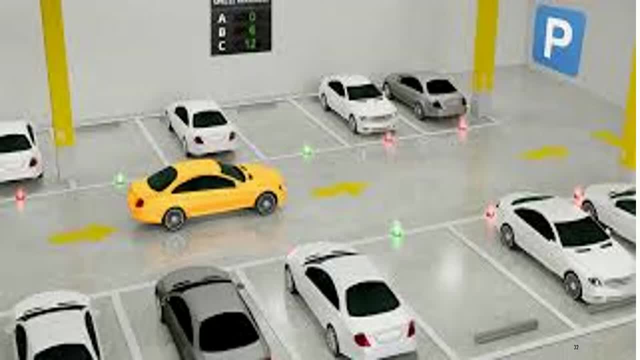 in a big bazaar, in the middle of the city or in a small bazaar, then we should be able to park our vehicles. so this type of parking also take care of us. so every time this point will be arise: the where to park our vehicles. so nowadays, um the private companies and private peoples are providing this. 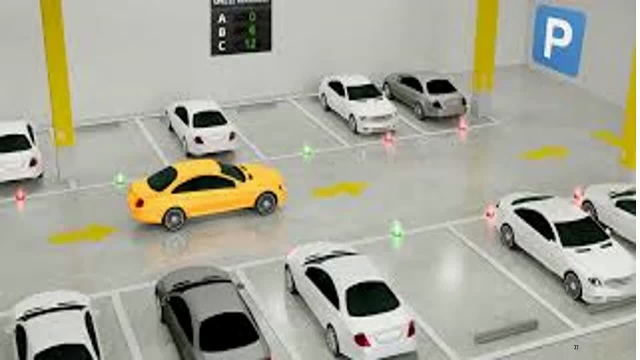 type of parking so that we can safely park our car there. and uh, there are various type of parking pattern. already we discussed that the car can be parked in 90 degrees, the car can be parked in 60, 30 degree or, and we know that parking may be parallel type of parking. parking may be: 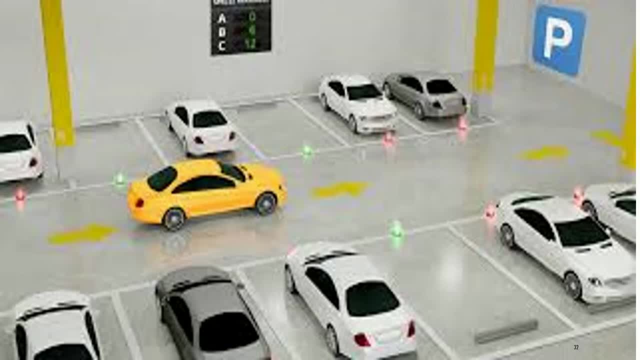 perpendicular type of parking. the main motto to use this type of various pattern for the parking is to reduce the space and in minimum area, the maximum parking should be available. so i hope, student, uh, you can understand uh, today's our concept uh, which is regarding or regarding to: 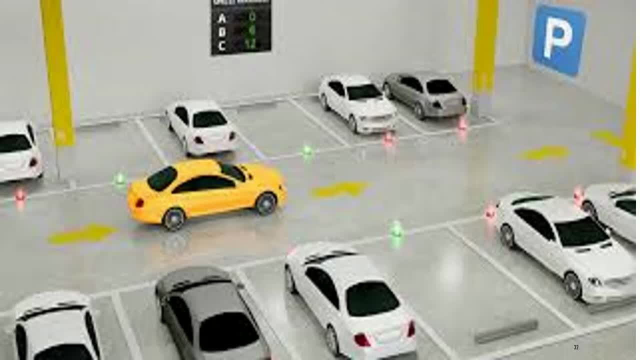 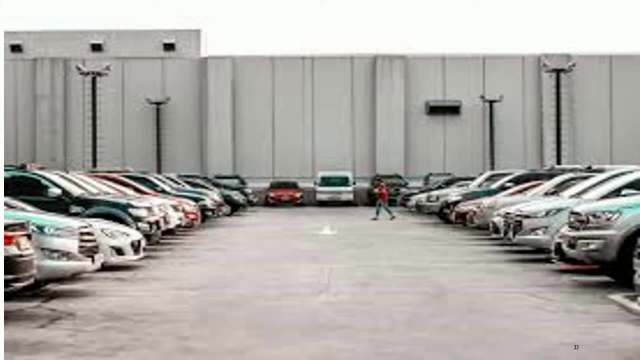 the parking. so in today's class mainly we have discussed about the. what do you mean by the traffic engineering? uh, also we have discussed about the three is of engineering, and then we discuss about the parking pattern. so there are various types of parking. uh, that parking pattern. 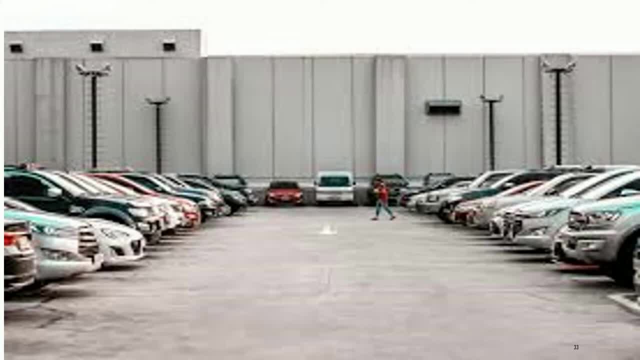 we discuss angled parking state or parallel parking. so, uh, in this figure, uh you can see, this is one uh industrial area uh where all the vehicles are parked uh to nose to each other. so this is also one of the parking type uh where uh each vehicle is perpendicular to each other. 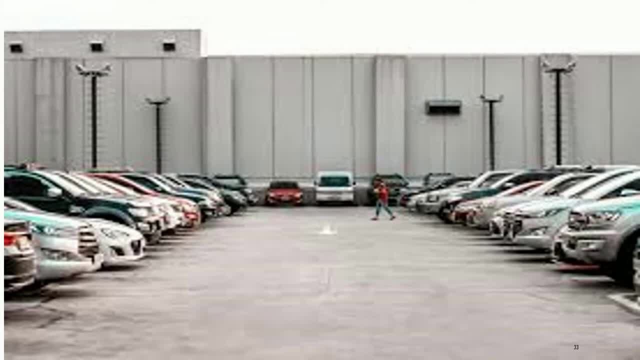 same time, uh vehicles are parallel to each other. so, as per the requirement of the site, the requirement of in uh industries, and as for the available uh open area, we are designing the parking. so these are the various uh parking slot. we already discussed about this parking slot. 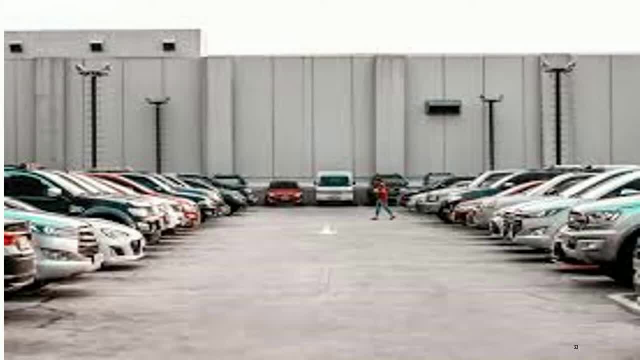 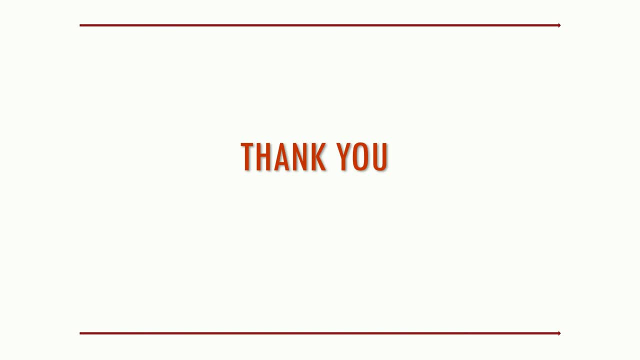 and, as per the requirement, we are providing this parking. so, student, i hope that in today's class, the point, uh, those we have discussed, uh, you may uh understand. uh, basically, we discuss about the three's of engineering. we also discuss about the. what do you mean by the traffic signal? what are? 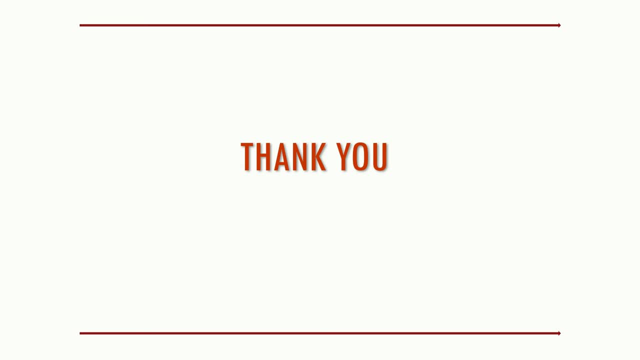 the importance of traffic signal. what are the various types of sign, why one should follow this signs and signal? because following the traffic rule is a psychological uh behavior. but if you want to reduce the road accident in india, everyone should follow all these uh traffic rules. he should follow all sign and signal which is beneficial for us and our future generation.